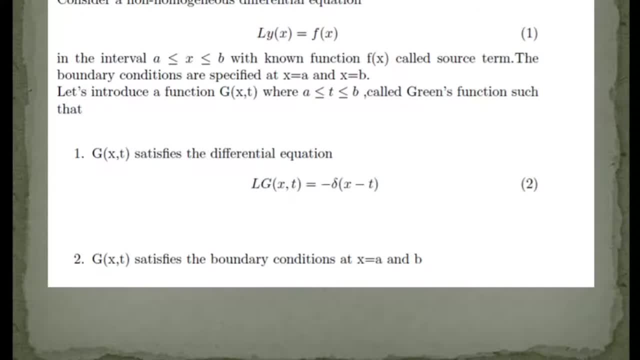 g, x, t is our Green's function, Okay, and the t is a sum value which is between a and b. t is a sum constant value which is lying between a and b. That is, a less than or equal to t, less than or equal to b. 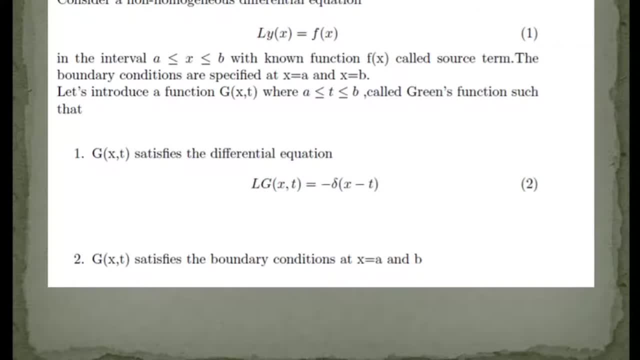 So this g, which is a function of x and t, g of x, t is called the Green's function. We cannot take the Green's function for granted. The Green's function should satisfy certain conditions. Okay, so the Green's function we have chosen is the first condition. 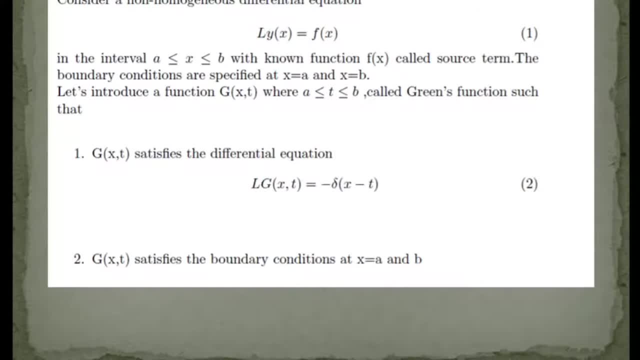 That is, if your operator l is acting on g, you should get minus of delta x minus t. Okay, so condition that we should choose g in such a way that l acting on g of x t will give minus of delta x minus t. 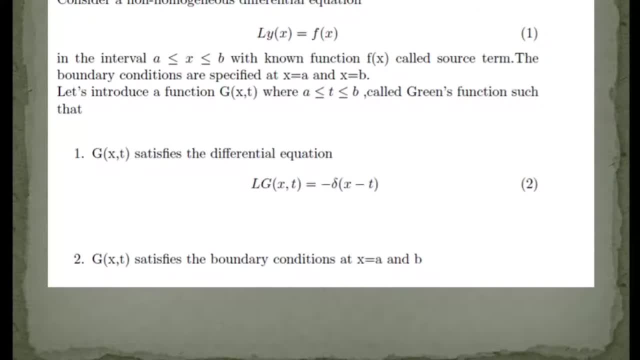 Okay, and also g of x, t satisfy the same boundary condition at x equal to a and b. Okay, these two conditions satisfy g. Now g, that is l. So initially in equation number 1, the operator l, that is l, g. acting on g, you get the delta function. 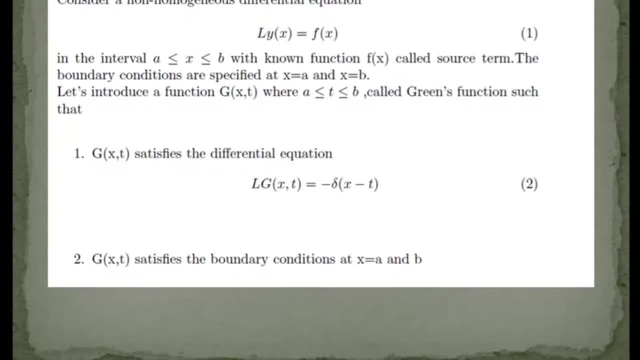 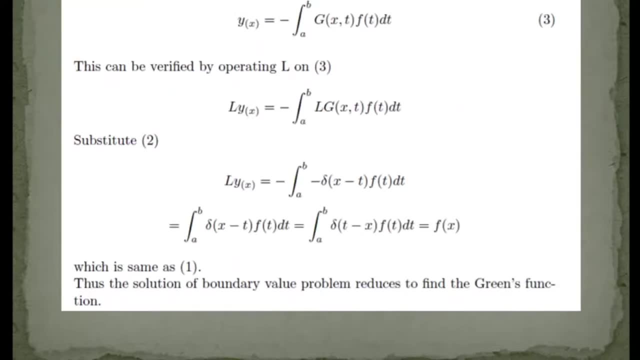 At the same time, g should satisfy the same boundary condition of y at two different points. Okay, now we are assuming a solution In equation number 1, we assume that y of x equal to minus of integral a to b, g, x, t, f of t, d, t. 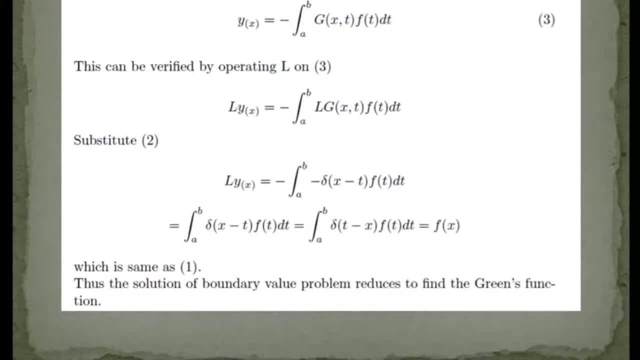 Okay, g of x, t at t is f of t. so integral minus of integral a to b, g of x, t, f of t d t is the solution of this equation. If you operate equation number 3 with l? l in equation number 3, we will get l? y of x equal to minus of a to b, l. g of x, t, f of t, d t. 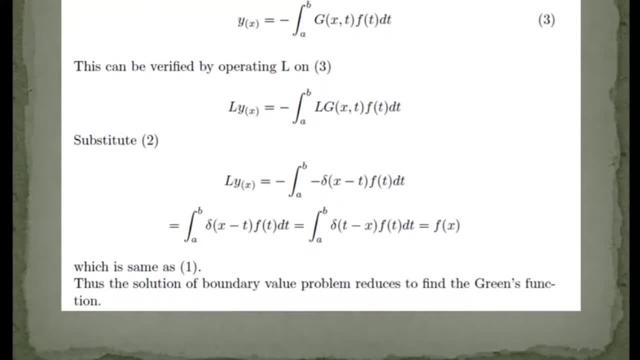 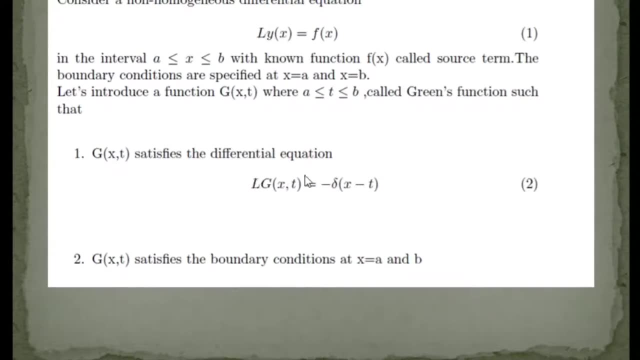 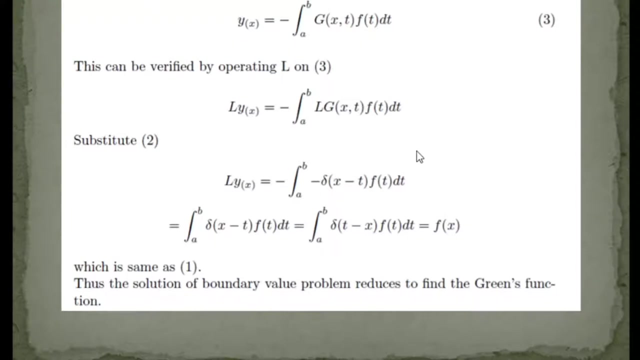 Okay, now equation number 2, this is our equation. Sorry, this is our equation number 2, l g of x, t is our equation number 2.. And that equation number 2, if you substitute on this one, so you will get l y of x equal to l, acting on g, l g of x, t, f of t. 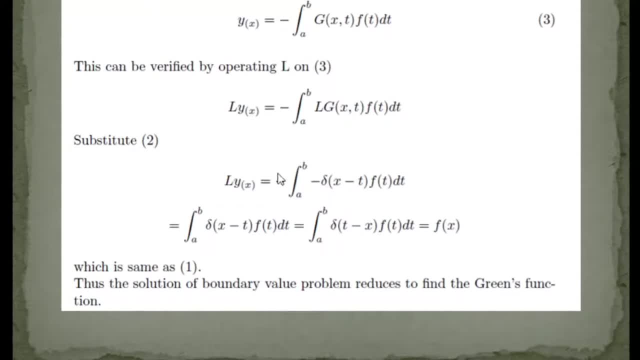 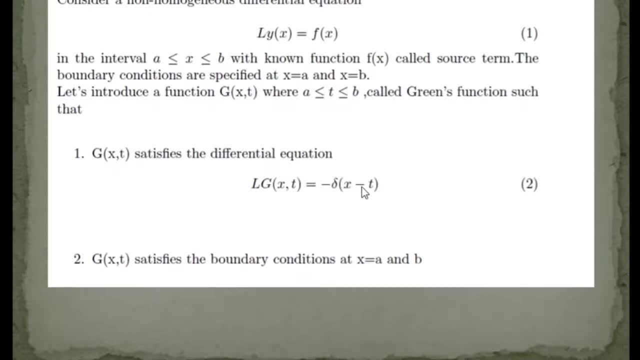 So substitute equation number 2,. if you substitute, you will get l y of x equal to minus a to b, l g equal to minus of delta i of x minus t And equation number 2, so that is my this: l g can be replaced with minus of delta x minus t, f of t d t. 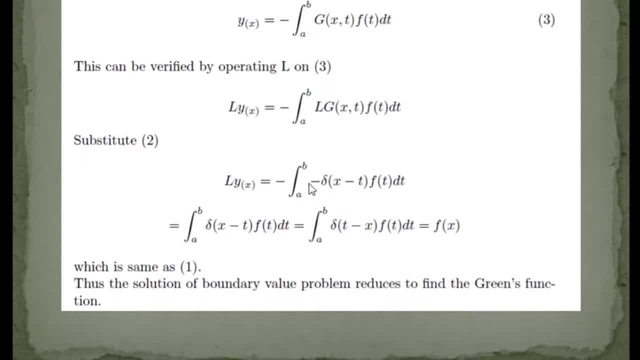 So a to b minus and minus become plus a to b. delta i of x minus t. f of t d t. We have seen before: f of x minus t is equal to delta i of x minus t is equal to delta i of t minus x. 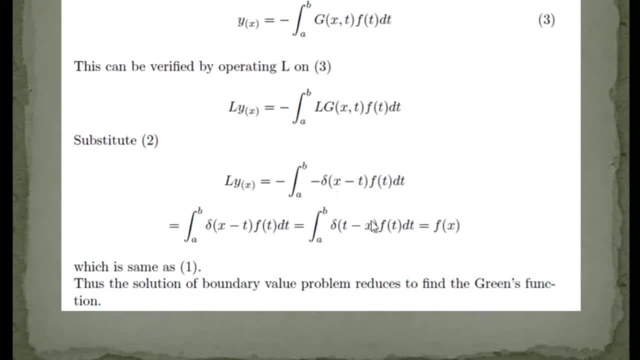 So this equation will reduce to f of x, Delta i of t minus x. f of t d t will be equal to f of x. Okay, so that means l y of x is equal to f of x. So our, our assumed solution, y is equal to minus integral a to b, g of x, t. f of t d t is the correct solution which we can cross-verify. 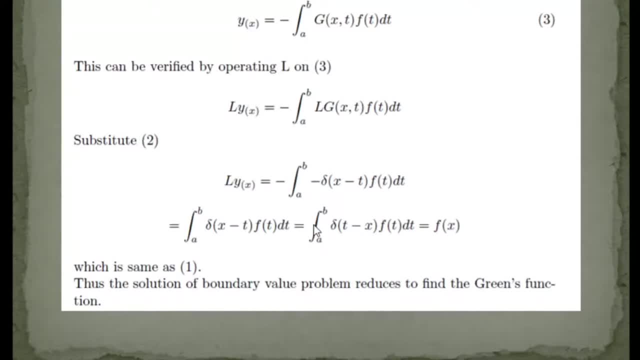 So, to put it short, our boundary value problem, if we want to find a solution in a differential equation, we can find that solution in the form of Green's function, that is, in equation number 3.. And so we can find the Green's function. 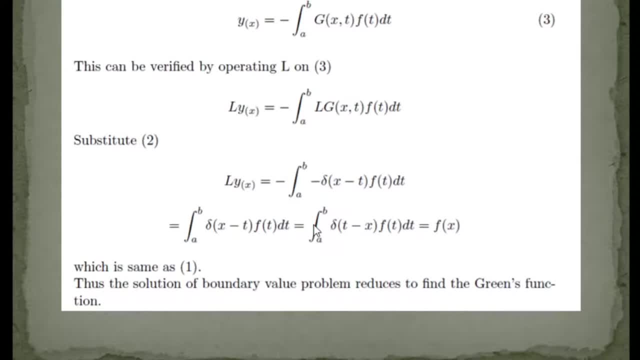 If we were able to evaluate that, we can easily find the Y for Y, that is, we can find a solution in a differential equation. So, in effect, our boundary value problem is: it is simply reduces finding out the Green's function for that particular problem. 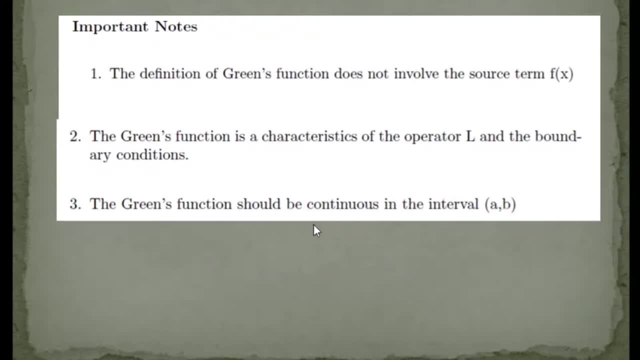 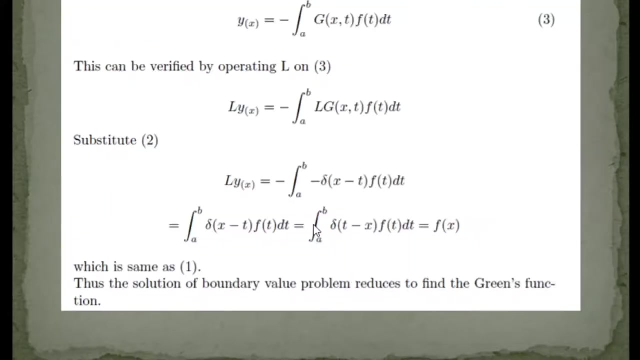 Okay. so to understand these integration�s, there are two things. the important one is not so. no one definition of the Green's function does not involve a source case. The f of x is not them means functional definition. one of them, okay, G, is the definition of the film. 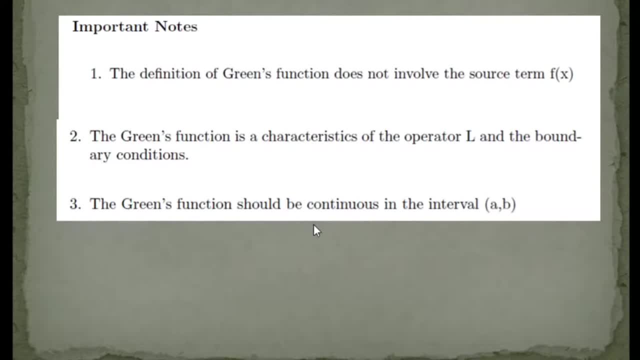 but it's not a definition of the institution, does not involve. so it's time of office, which means. number two means function. is this simple characteristics of your operator and bounty condition. number two means function, depending on the way you do cut a gun when you are in other, it is the. 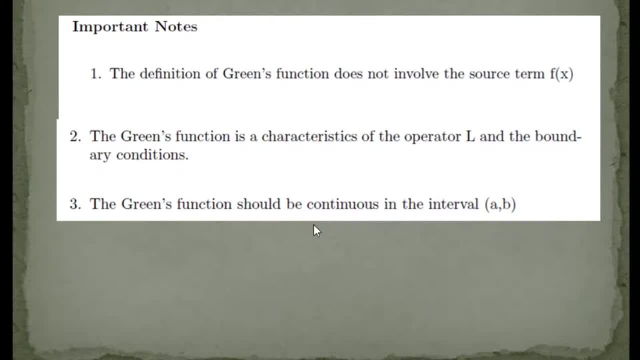 operator, whatever be the operator and also the bounty condition. so it means function, it is a characteristics of the operator and the bounty condition. it's not at all depending upon the source stem, and the third condition is that it should be continuous in the interval. now let us try to find out the means. 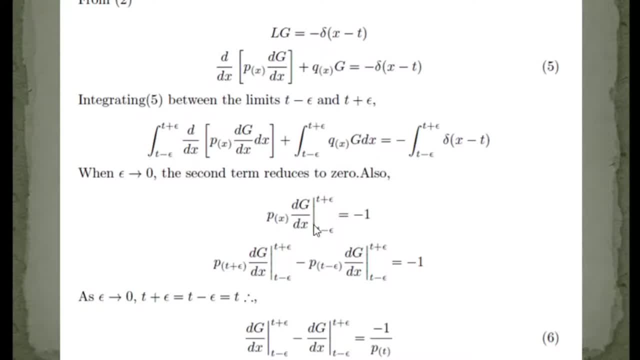 function for the one-dimensional. so let us for that number number on the SL operator at the general SL operator, that is, n is equal to D by DX of P of X, D by DX of Q of X. okay, number a. question number two. number one of the. 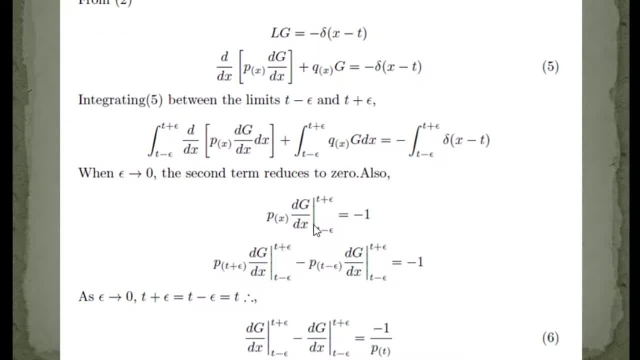 level of LG L acting on G is equal to minus of Delta X minus. okay, so now D by the X of so LG L in the water number two. question number four I would have substituted on in the new item is on over to substitute my D by DX of P of X. 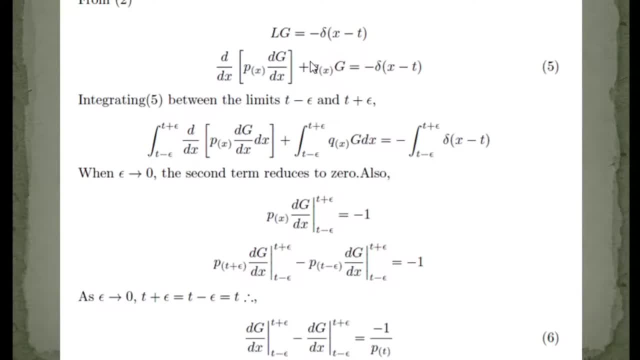 C by DX of G plus Q, G equal to minus Delta, X minus. okay, equation number two in a two lagging alien water operator, a subsidy number on the data. so now we are going to integrate between the limits T minus epsilon to T plus epsilon, so just. 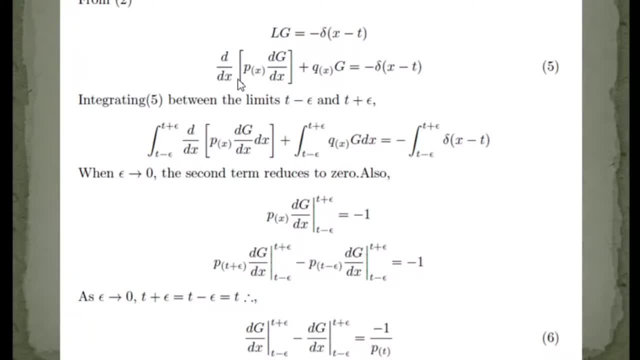 integrate on both sides. now the second time of canal. it is an integrating Q of X, G, DX. when we apply the limits T minus epsilon, T plus epsilon, we assume that epsilon is very small, so epsilon, epsilon tends to zero the upper limit and lower limit. when we apply this time, the difference time will be very, very small. so that can. 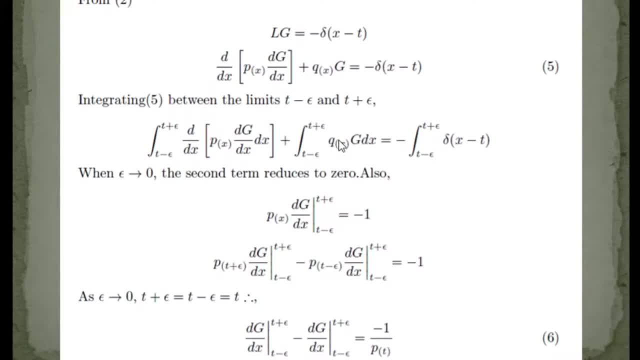 be assumed to be equal to zero. the Q of X- G, when we apply the limits T minus epsilon, T plus epsilon with epsilon 10 tends to zero this time will be very, very small, which is it can be approximated to be zero. that same approximation cannot be. 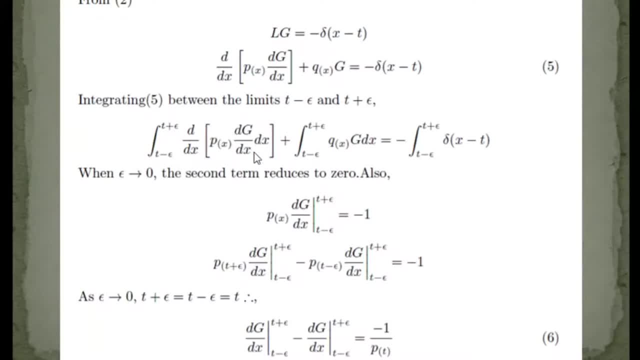 done here because it involves three differential times. okay, so the first time we integrate the integral and the differential time disappear. so this in general will give you the integration will give you T of X, D, G, body, X between the limit T minus epsilon, T plus epsilon, so the right hand side become 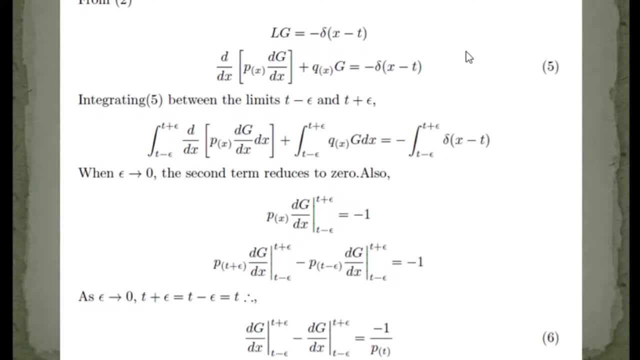 minus of integral T minus s epsilon T plus epsilon del tx- T a inlaimed, don't know. delta function integrated need not be always. comment is if you with the Duncan a, B, 4 range of independent can be team on a. но Benny Bennett are useless on произош between less. instead of this r a points. 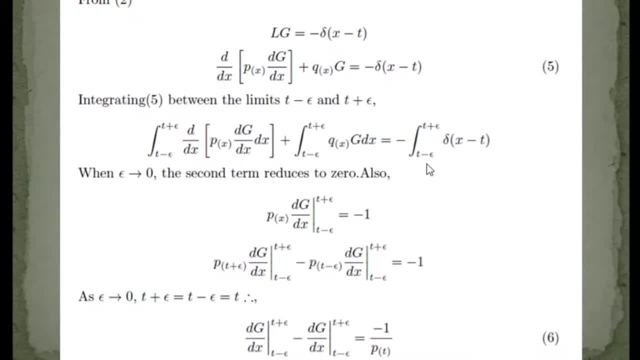 So this equation, this term will be reducing to this integral, with the dx integral minus integral, t minus epsilon, t plus epsilon, delta x minus t, dx will be equal to 1.. So this is equal to minus 1.. Now we apply the limits, limited limit value to p, that is, p of x become t plus epsilon. 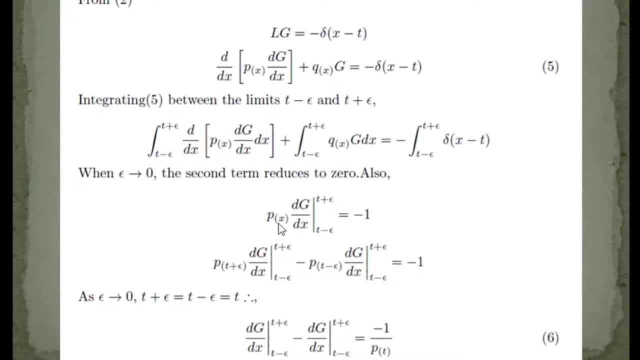 dg by dx between the limits p minus epsilon, t plus epsilon minus p, t minus epsilon, dg by dx, which means equal to 1.. So, as I said, epsilon tends to 0. epsilon 0 will equal t plus epsilon and t minus epsilon equal to t. if we write above the equation: dg by dx, t minus epsilon, t plus epsilon minus. 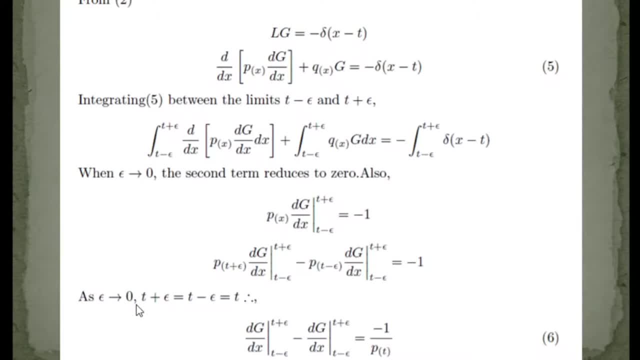 dg by dx, t minus epsilon, t plus epsilon will reduce to 1.. So this is equal to minus 1.. minus 1 by e of p. okay, so which means other quality. my parent, under the our deck around TN, were in a point in a difference in a continued master put: no. 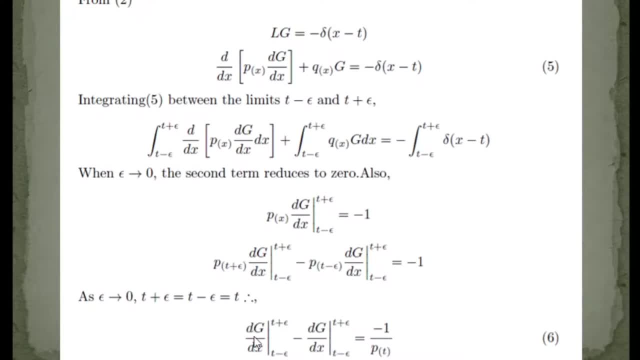 there is a discontinuity. there's a definite discontinuity for DG body X when we apply the limits. okay, first, differential of the games function has a discontinuity equal to 0- and I remember this committee. no continuity on the very much equal to 0 and there is a time minus 1 by p of p, which means there is a. 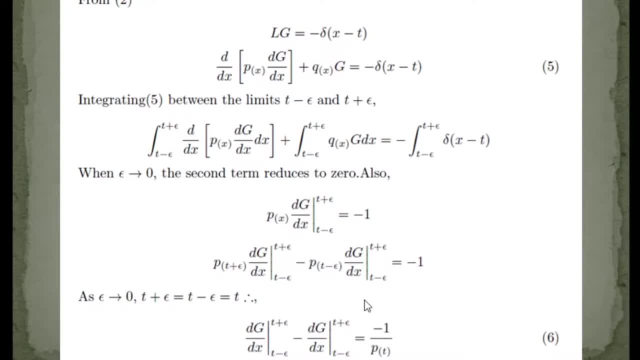 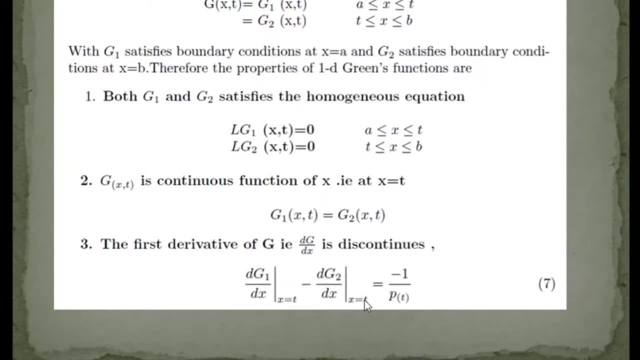 discontinuity for this DG by the X. so so when? so now I'm going to be number two: TN over in a point. around TN, epsilon tends to 0 around TN over in a point in order to means function, the first differential discontinuous on I'm gonna. 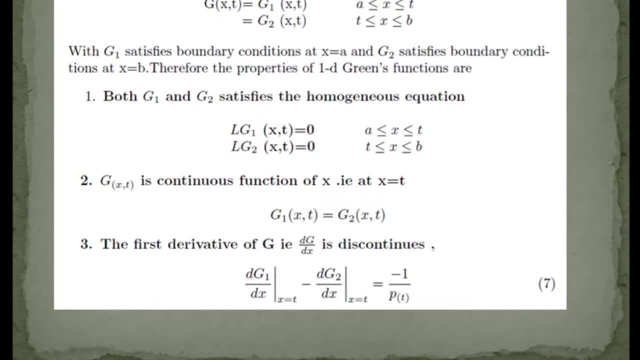 handle number two in the room, which means function a 215. oh yeah, to be an integer range, longer number to inspiration going to the consumer. can I write it with the very, because that is a discontinuity at the point P is completely in the first derivative. Okay, so the grains function is written as: G of XT is equal to G1 of XT and that will be valid from A to T. The second function is equal to G2 and that will be valid from T to B. 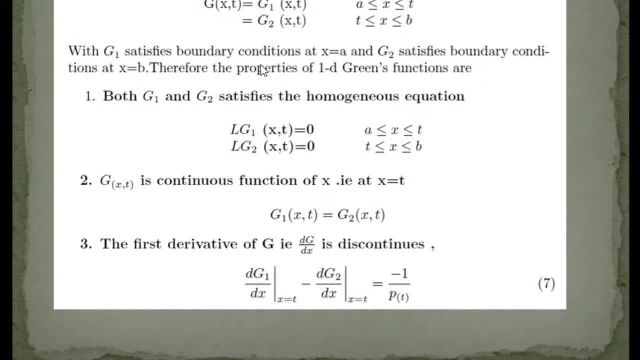 Okay, and G1 solution will satisfy the boundary condition of X, equal to A, but G2 will satisfy the boundary condition of B. This is the property of the grains function. So if we go to the property, we saw that there are two equations. So G1 and G2 will satisfy our homogeneous equation. 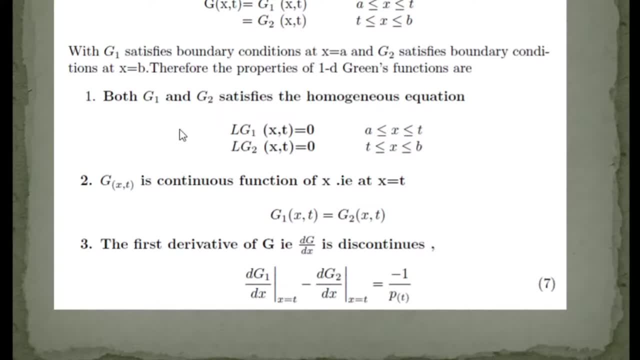 G1 of XT is equal to 0 between the limit A to T and G2 of XT is equal to 0 between the limit B to D. Okay, but at the same time, that is, G1 of XT is equal to 0 and G2 of XT is equal to 0, which means G is continuous at X equal to D. 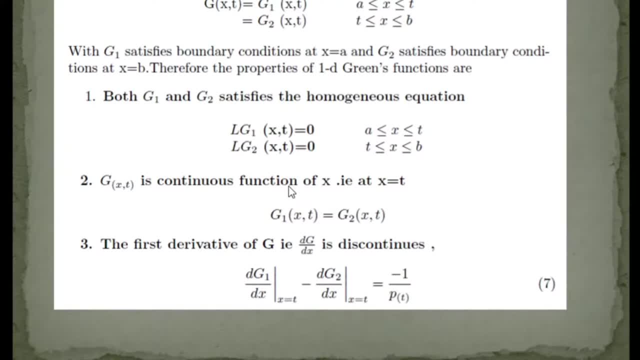 If G is continuous, the first derivative will be discontinued. So this is one property. G is continuous At X equal to T. at X equal to T, the value of G1 and the value of G2 will be the same. 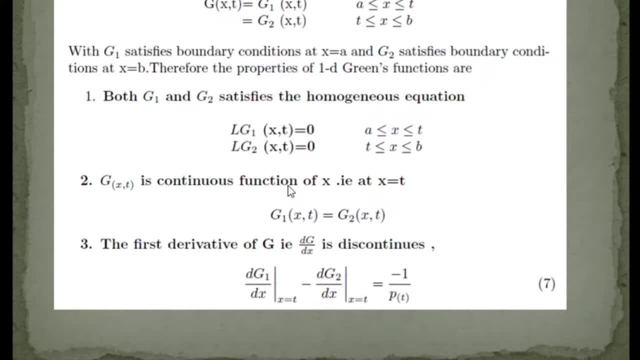 Okay, if G1 of XT is equal to G2 of XT, then there is two different. two grains function will have the same value at the point X equal to T, But at X equal to T point, the first derivative, G1 at X, DG1 by DX at X equal to T, minus DG2 by DX at X equal to T, is discontinued. 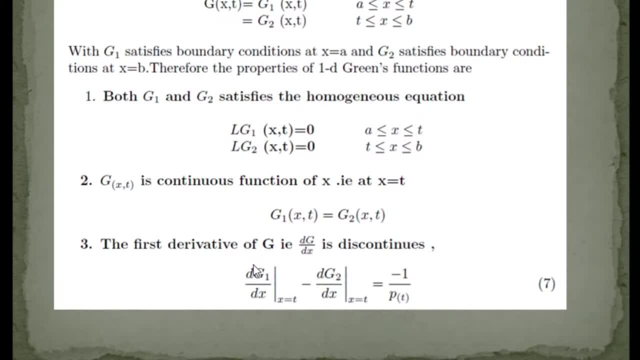 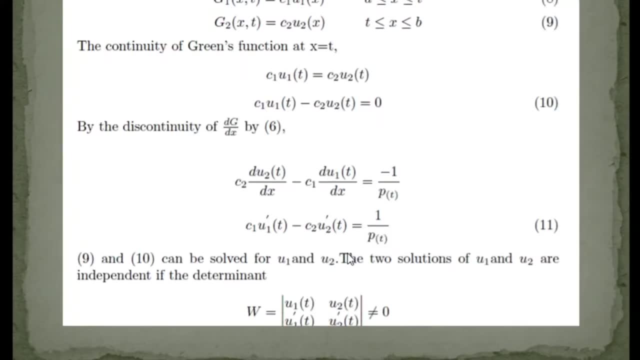 It is continuous and discontinued, So the discontinuity is measured by the quantity minus 1, by T of X. Okay Now, what do we want to know about G1 and G2?? We don't know what G1 and G2 are. 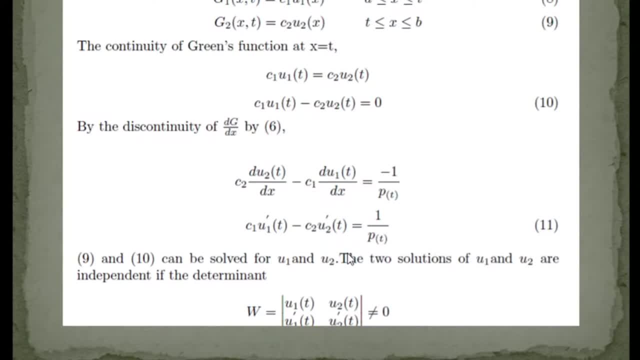 What is the G1 error? What is the equation of G1 and G2? Now let us try to evaluate this G1 and G2.. For that we assume that G1 is equal to C1- U1 and G2 is equal to C3- U2.. 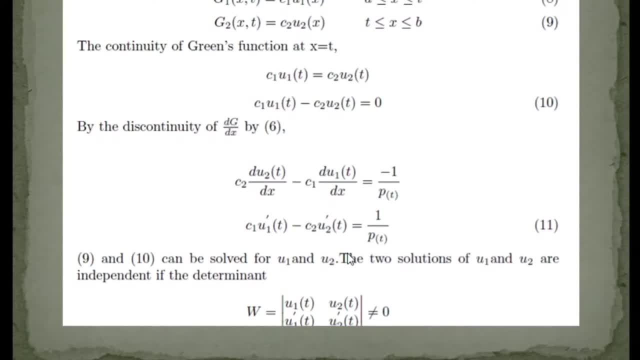 Now, at the point of discontinuity, we will write it as at the point X equal to T. So at the point X equal to T, this function is divided by 2. So at X equal to T, we can write G1.. 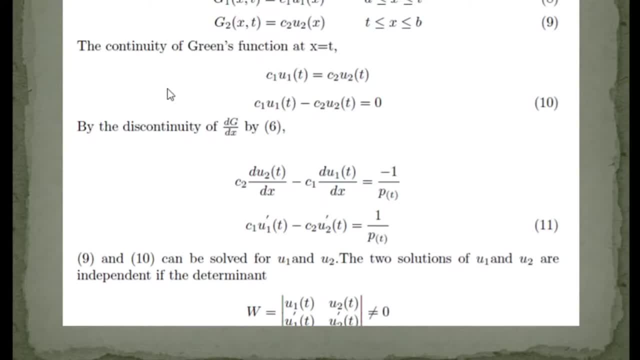 We have already said that Green's function is continuous at the point X equal to T. So we can write equation number 8 and 9 as C1 U1 at X equal to T. That is C1 U2, U1, T equal to C3 U2.. 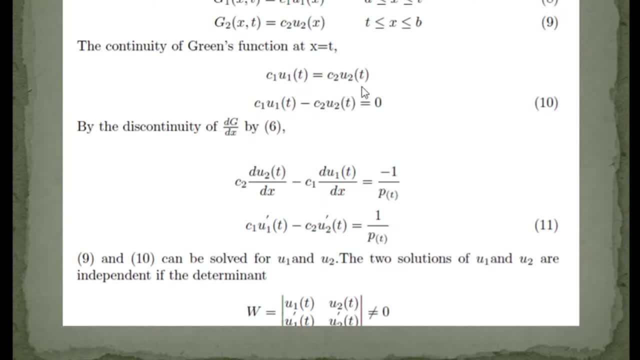 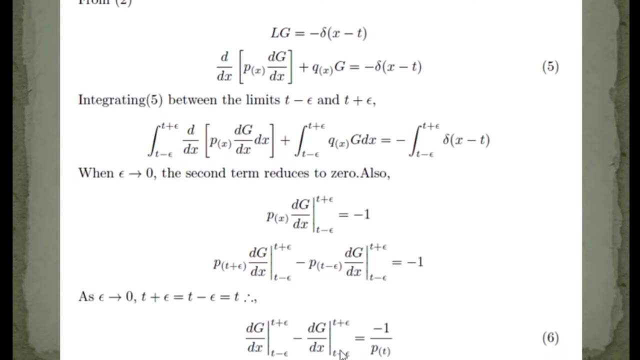 And similarly, so that we can write it as C1 U1 T minus C2 U2 T, equal to 0.. Now we have already said discontinuity, So discontinuity, this shows a discontinuity, So we can specify discontinuity like this: 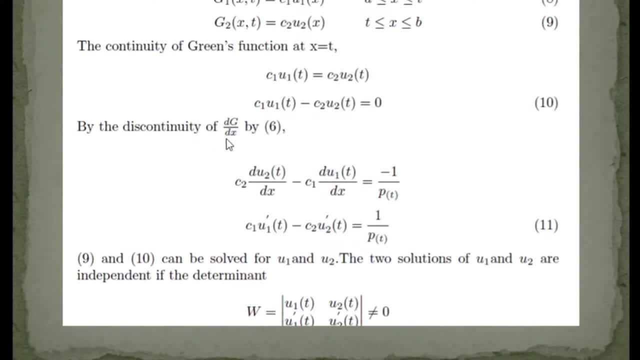 Discontinuity is: if we differentiate this one with respect to X, then at T is equal to T, we will substitute the value, So discontinuity is like this. So discontinuity can be written as C2, differentiate C2, that is, differentiate G2 with respect to X. 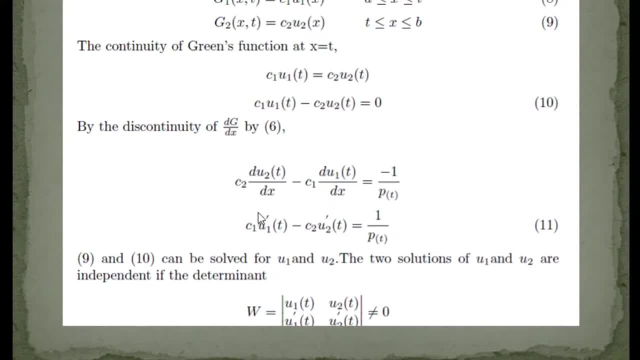 that is C2, DU2 by DX minus C1. DU1 by DX equal to minus 1 by PT at T is equal to T. So we have DU2 by DX at T and DU1 by DX at T and minus 1 by T of T. 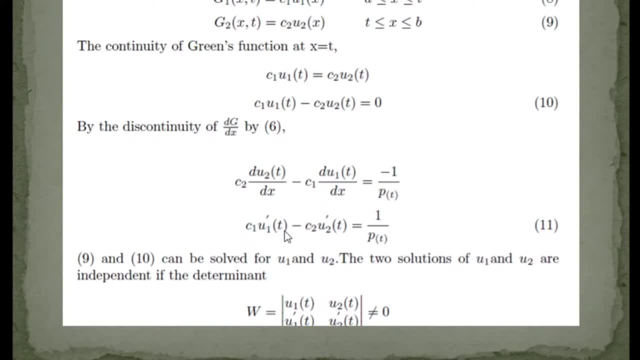 So I will write it as C1- U1 dash. C2- U2 dash. Since we have to remember that it is at T, do not write it as X. The discontinuity is at the point where T is mentioned, So we have to mention the point where T is mentioned. 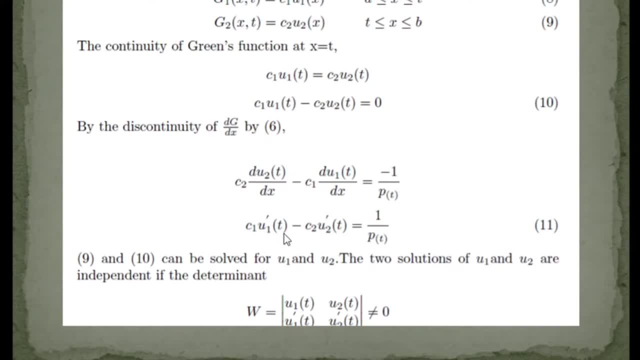 Do not write it as C1 U1, dash. Do not write it as C2, C1 U1, dash T, Since the discontinuity is at the point where T is mentioned. Okay, So here 9 is wrong and the equation number is 10 and 11.. 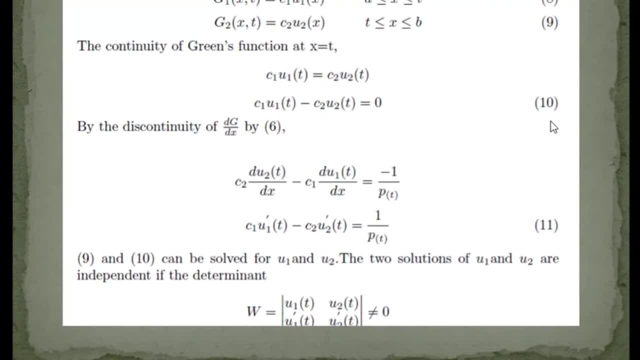 So we can solve between 10 and 11, equation number 10 and 11.. Then we can find out U1 and U2 by solving this. Okay, So solution of U1 and U2 are independent. This is a property that we do not know. 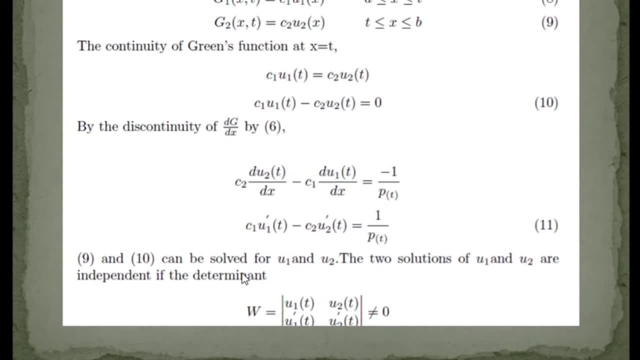 Let us take it like this. So the solution 2 of this equation, 10 and 11, are independent If the determinant of that is U1 and U2.. If it is independent, if the determinant is not equal to 0.. 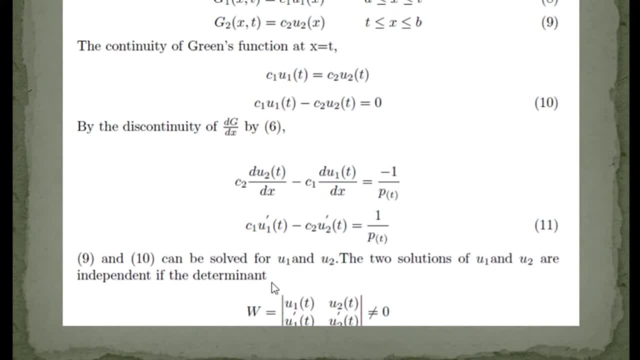 Okay, In this determinant where the equation lay U1, then random to equation U1 dash, that is U1 T, then U2 T. first equation lay 100 times first row lay. second equation lay 100 times U1 dash. 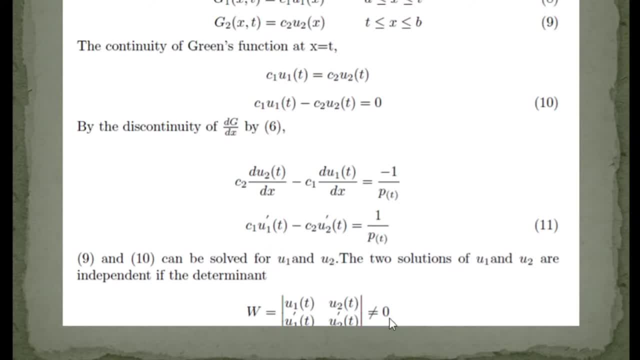 U2 dash not equal to 0.. Okay, So this is not equal to. if this determinant is not equal to 0, we will have. we will have two independent solution. Okay, This determinant is called a Wronskian. 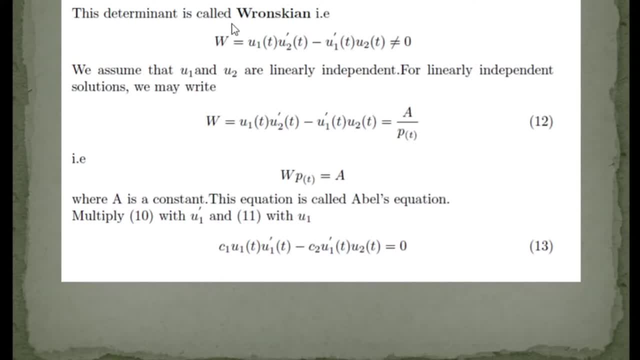 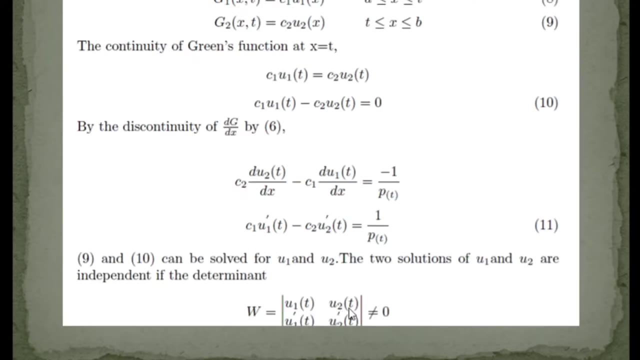 Okay, That is denoted as W, So Determinant. expand here. So: U1 T this U1 T, U2 T dash minus U2 T, U1 dash T. Okay, This is not equal to 0.. 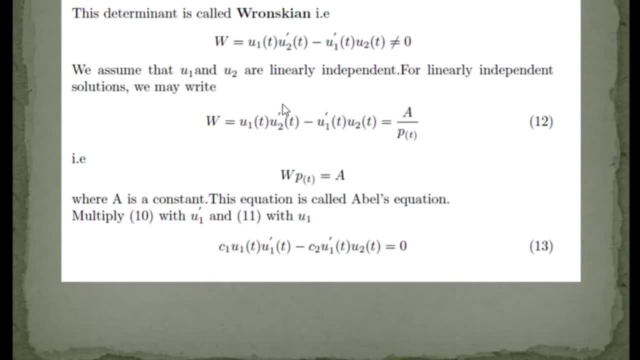 So, since we are assuming that U1 and U2 are two linear, two independent solution and this W can be written as A into T by T, A, A divided by T, T, T, T can be written as this determinant equation: 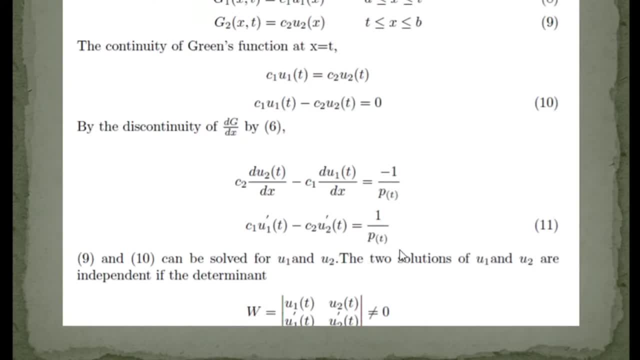 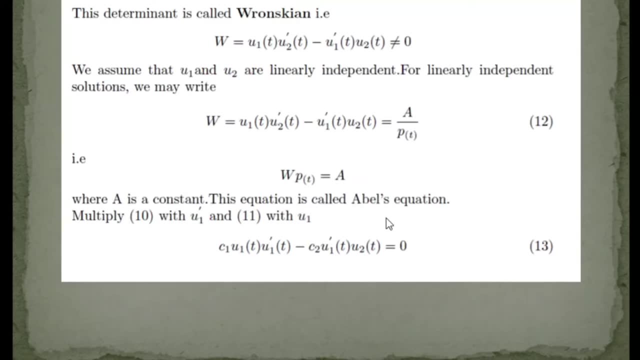 1 by T T, 1 by T T into some constant- Okay, Right answer is equal to 1 by T T into some constant, So W. so you can write it as W. W into T. T is equal to A. 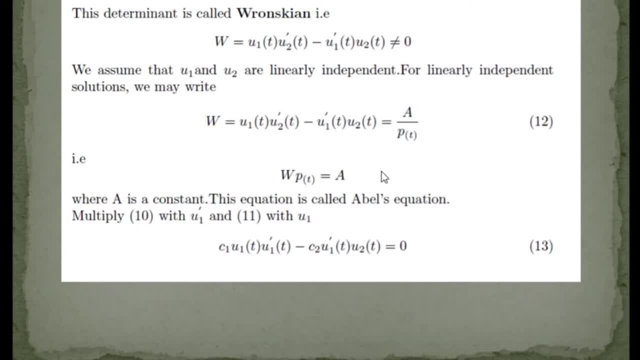 where A is a constant, and this equation is called Abel's equation. Okay, Now we have found C1 and C2, and now we have come to the solution. So equation number 10,. this is equation number 10,. 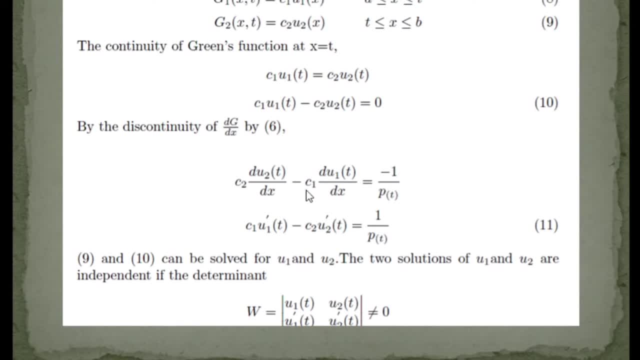 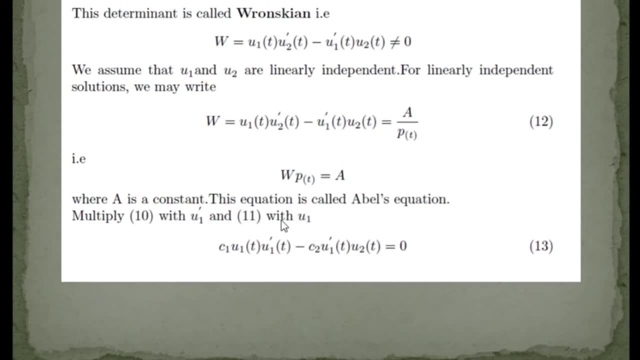 and this is equation number 11.. So multiply equation number 10 with U1 dash. Okay, Multiply equation 10 with U1 dash and equation 11 with U1.. And just simply do the math: C1, U1, U1 dash. 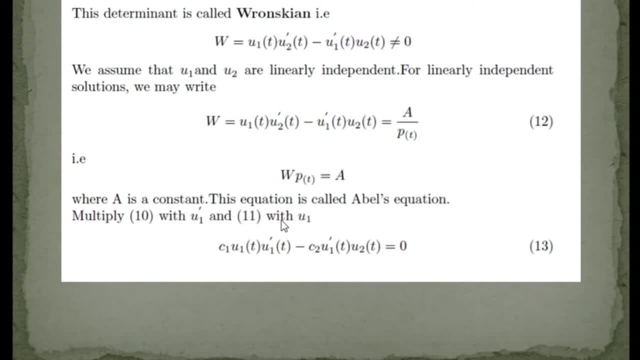 minus C2, U1 dash, U2, equal to 0.. And the second equation: multiply with, multiply with U1, and you can write it like this: Okay, This equation, equation number 11.. Equation is: U1 dash. 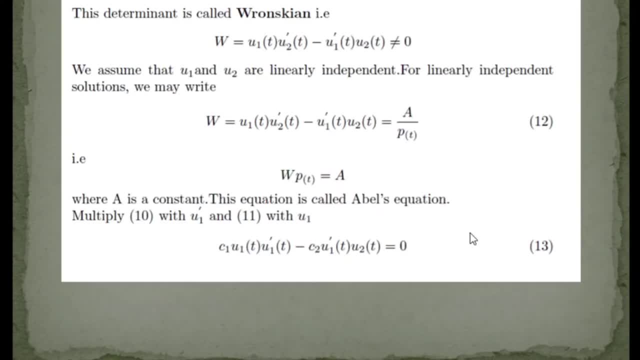 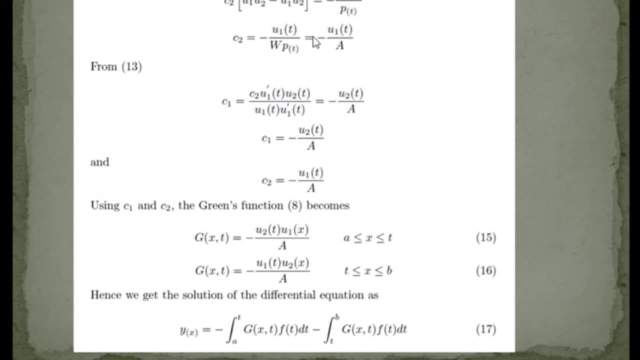 and now the equation is: you want to multiply with. you will write it like this: So then I take the reference equation 13 minus 14, you will get, and solving this one, you will get C2.. C2 in the equation is: 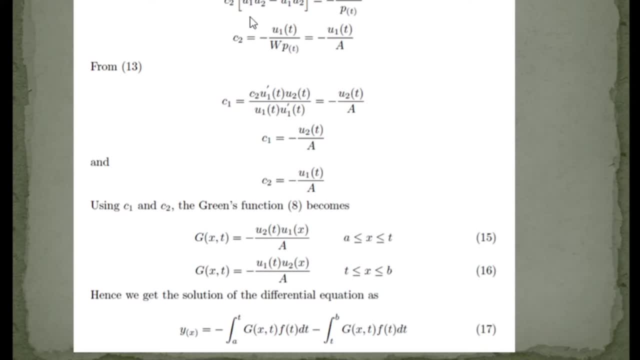 you will write it as W. C2 into W is equal to minus U1 by T T. So C2 is equal to minus U1, T by W into T, T. W into T, T is A. we have defined W into T, T equal to A. 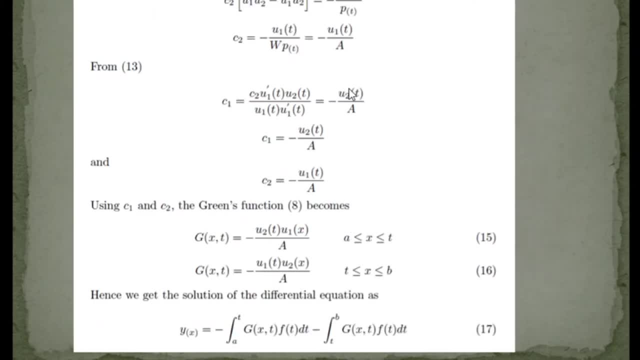 So this is equal to A. So similarly from 13,. if you substitute this C2 here, you will get the value of C1.. So the value of C1, the value of C1, we can solve this easily. 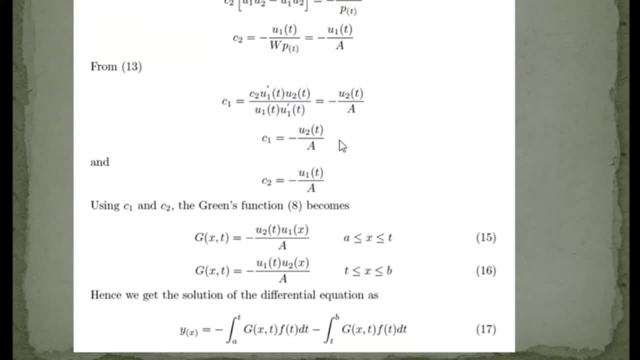 The value of C1 minus U2 T by A And the value of C2 minus U1 T by A. Remember here the key: the x should not change. Then when we write T, u2 T, we have the constant value there. 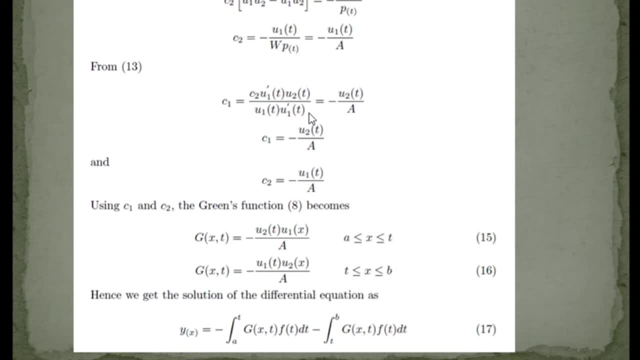 U2 T plus 1 T plus u2 T is the value of a specific function, not just some variable. So if we substitute this C1 and C2 against function like this, we will get this equation. the first equation is the solution we had for assigned agents. 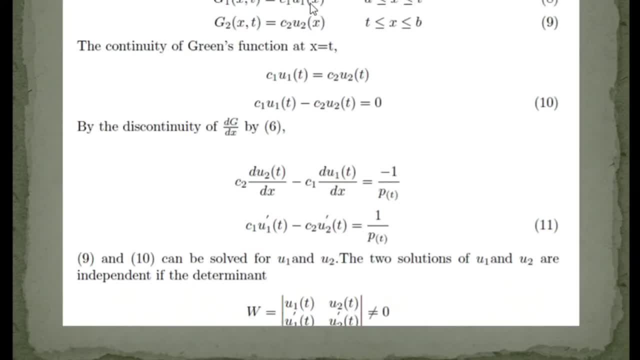 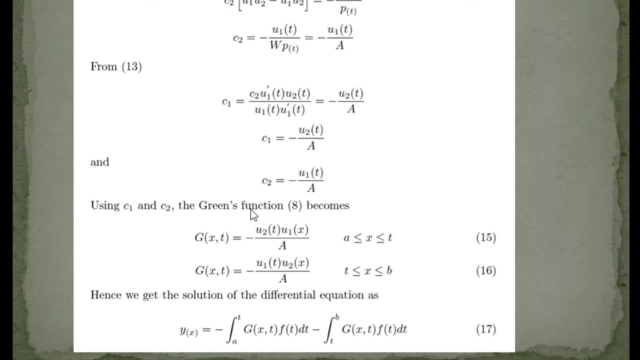 G1 is the value of C1 into U1 of x and G2 is the value of C2 into U2 of x1. So we got C1, we got C2.. So let us exclude equation number 8 to 9.. So here G is equal to C1 minus U2T by A. So U2T by A into U1 of X. and second equation- sorry, second equation- minus of U1T into X by A.